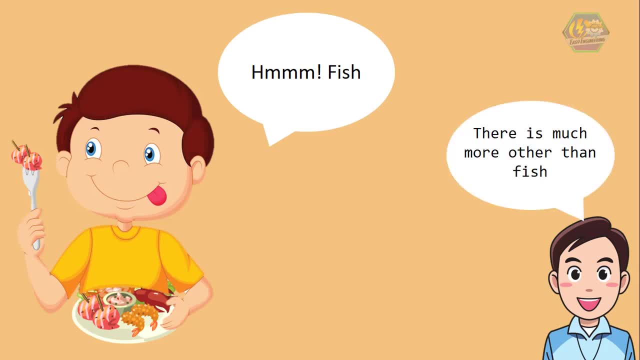 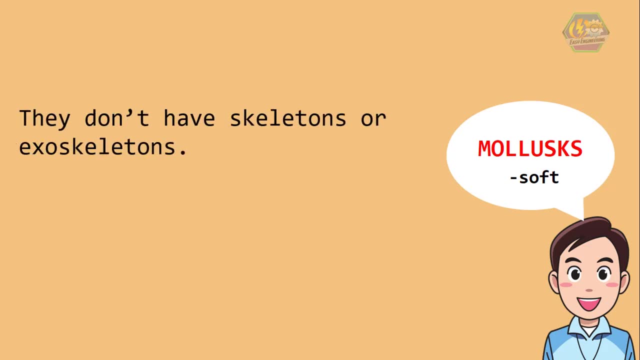 But there is much more other than fish, and some of them belong to a class of invertebrates called the mollusks. The word mollusk means soft. They don't have skeletons or exoskeletons. Some have shells made of calcium. 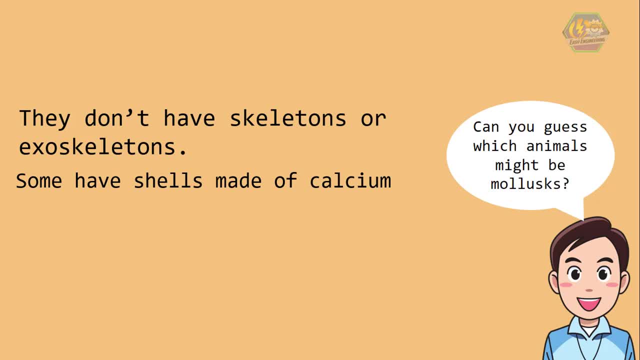 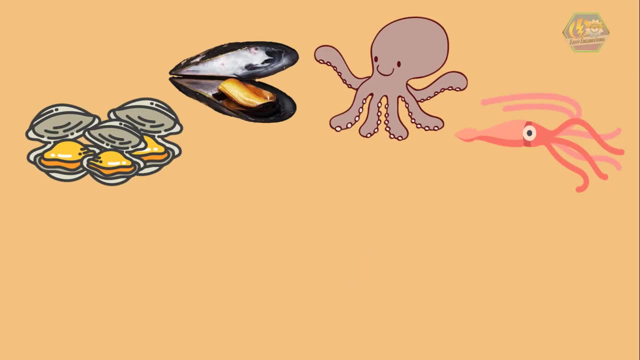 Can you guess which animals might be mollusks? If you guessed slugs and snails, you are right. Clumps, mussels, octopus and squids are also mollusks. Think about it: None of these animals have bones, They are all soft. 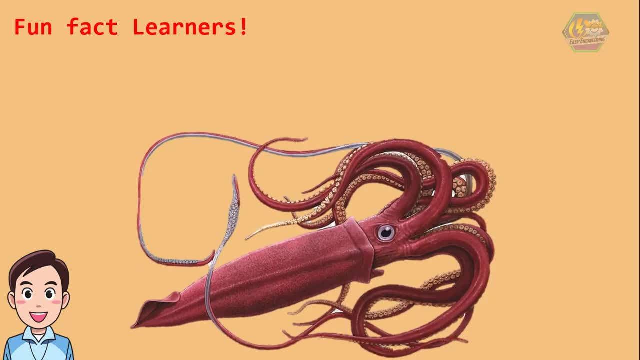 Fun fact learners. did you know that there are monstrous squids? Most squids are small, but the giant squids can grow up to 55 feet long- That's like three buses long- And their eyes are the size of beach balls, which lets them see in the dark ocean. 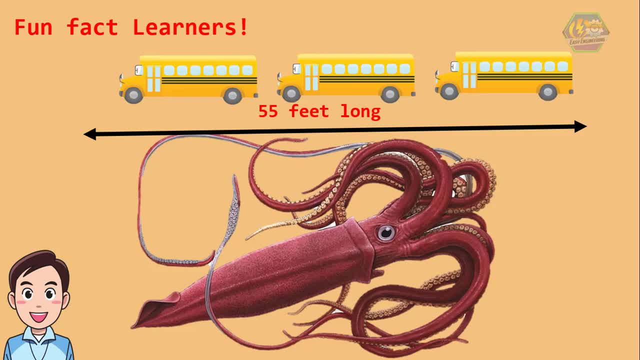 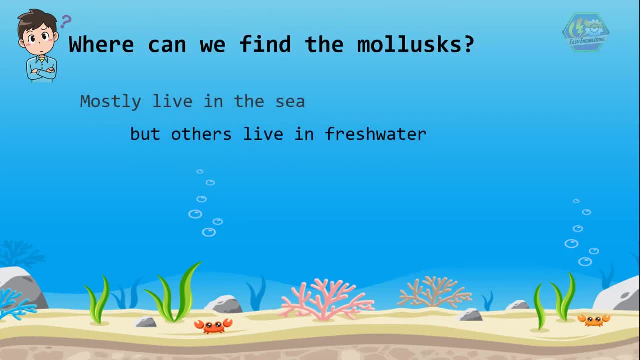 Most of the ocean deep haven't been discovered yet, so there could be something bigger. Now where are the mollusks? Where can we find the mollusks? Mollusks mostly live in the sea, but others live in fresh water. 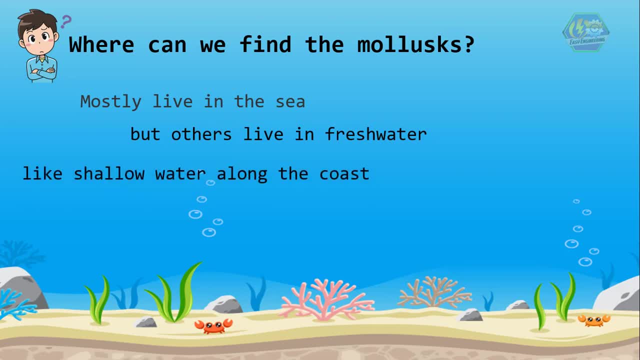 Some like shallow water along the coast. If you dig up some sand on the beaches you can find many of them. They are abundant and very delicious. Many mollusks, like the clumps, dig into sandy or muddy bottoms. Others prefer deep water, like the squids. 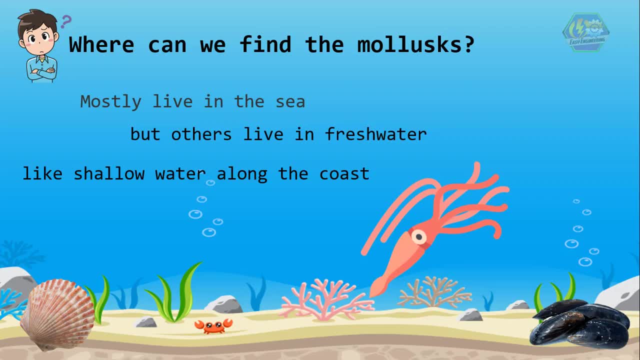 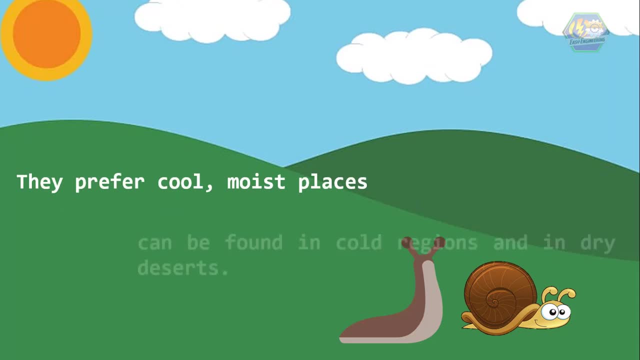 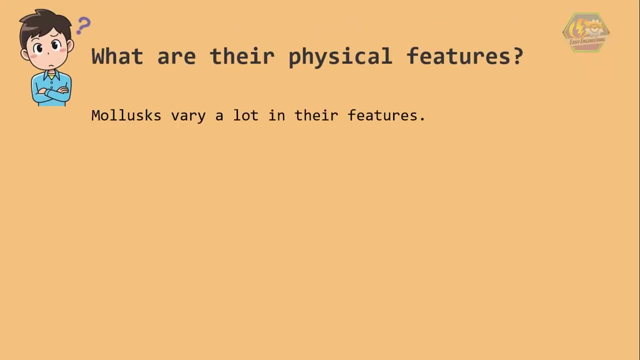 Some attach themselves to rocks in the ocean, like the mussels, Some snails and slugs. They prefer cool, moist places, but they also can be found in cold regions and in dry deserts. What are their physical features? Mollusks vary a lot in their features. 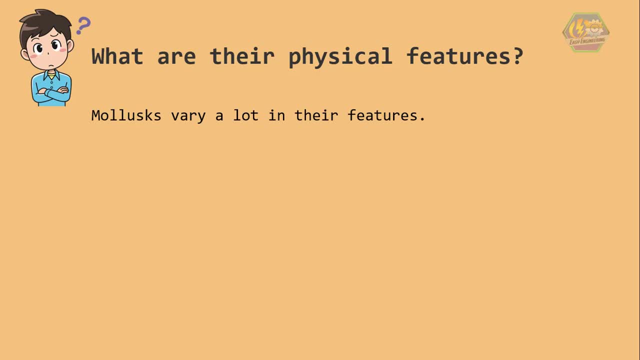 Even mollusks of the same type can be very different. like the squid, Some are small like the ideate tip of your finger and some are monstrous. Basically, they have a soft body that holds the heart, liver, digestive system and other important organs. 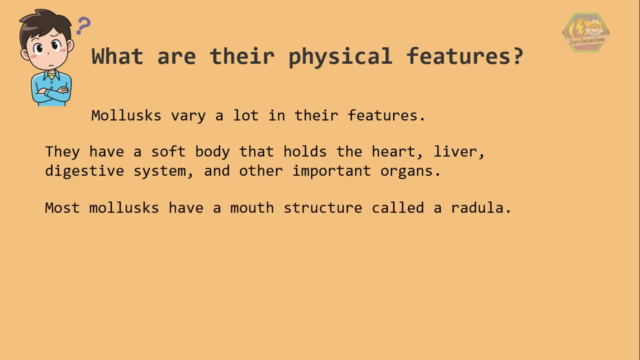 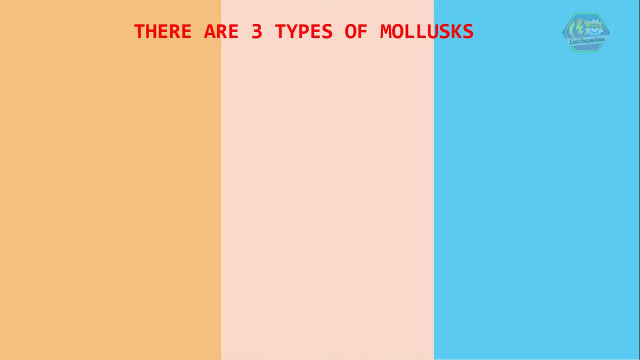 Most mollusks have a mouth structure called a radula. The radula is sort of like a rough tongue with lots of tiny teeth. There are three types of mollusks. Gastropods are the snails and slugs. They use their foot to crawl. 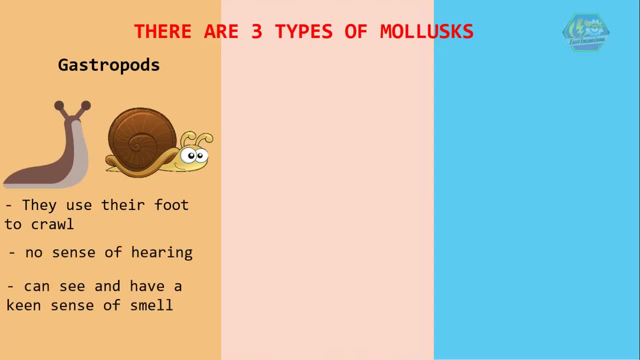 They have no sense of hearing, but they can see and have a keen sense of smell. Bivalves include the clams, scallops, oysters and mussels. As their name implies, they have two parts of their shell Which can open and close. 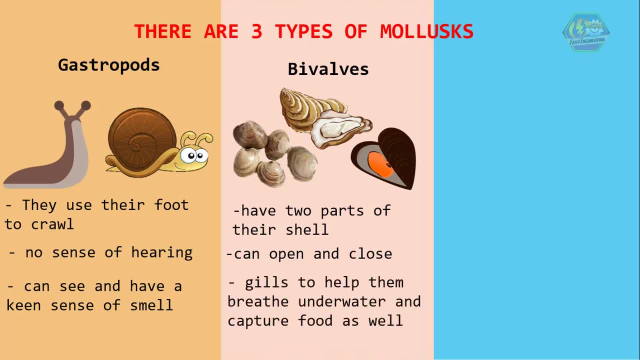 They also have gills to help them breathe underwater and capture food as well. Oysters are some of the most delicious seafood. Cepalopods are the octopuses and squids. They have a set of arms or tentacles. They can also camouflage or change color for defense. 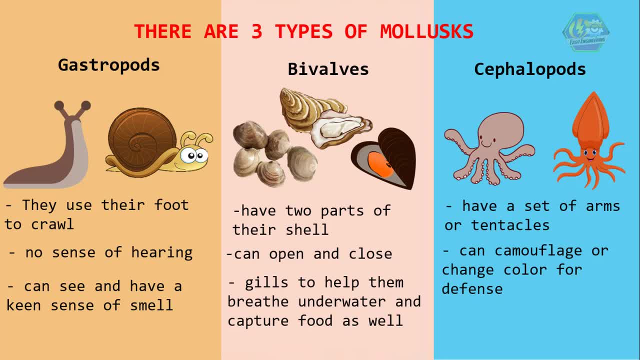 They can also squeeze through a coin-sized hole. Cepalopods have three hearts that pump blue blood And they are thought to be the most intelligent. They are also known as the most intelligent of invertebrates. Someday they could challenge us. 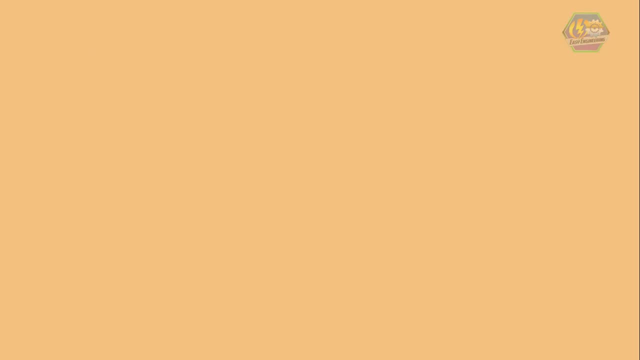 Who knows? Most mollusks with shells have a foot. The foot moves them forward by expanding and contracting muscles. Clams also use this foot to dig up or down the sand. It is just called foot because it is just the one foot. 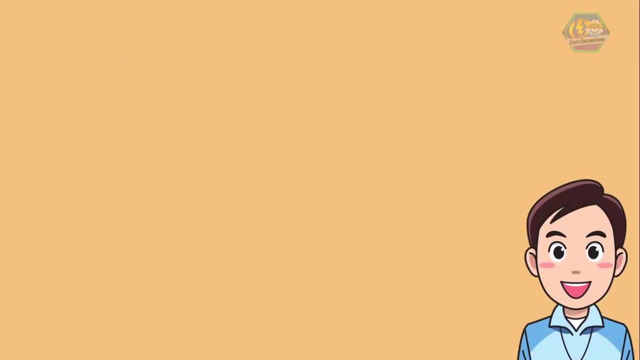 Not like us that have two feet. Fun fact learners. Did you know that some oysters can alternate their gender? That means they could be male in one year. That means they could be male in one year. That means they could be male in one year. 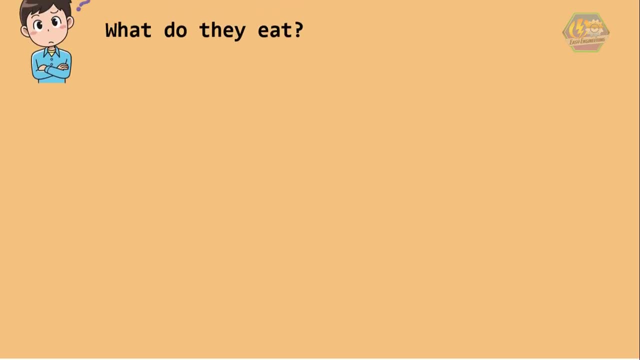 And female in the next year. Now, what do they eat? Many mollusks eat mostly algae. They use the radula to scrape algae off rocks. Snails and slugs eat plants and fruit. On the other hand, an octopus can go after prey as large as a shark. 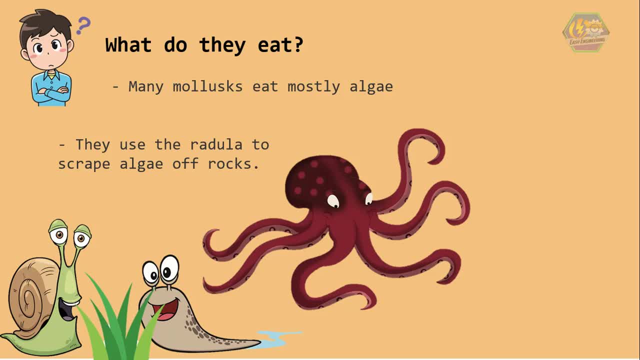 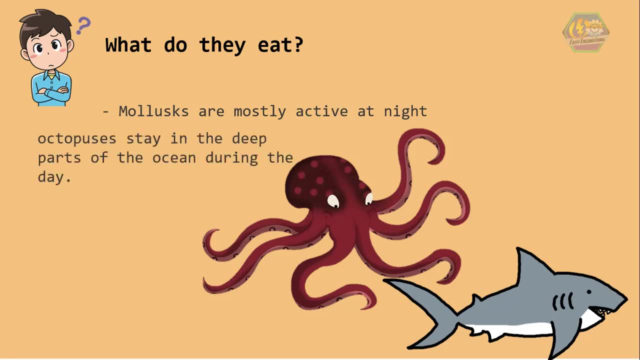 On the other hand, an octopus can go after prey as large as a shark. How fearless Mollusks are mostly active at night. In fact, octopuses stay in the deep parts of the ocean during the day. In fact, octopuses stay in the deep parts of the ocean during the day. 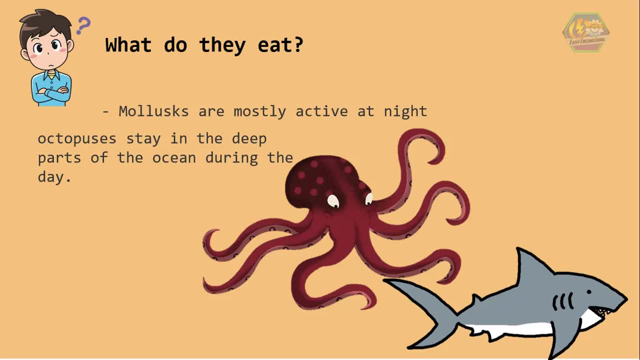 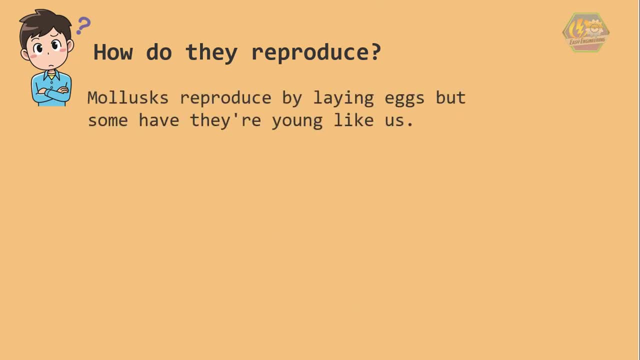 At dawn and dusk they swim closer to the surface. At dawn and dusk they swim closer to the surface for something to eat. how do they reproduce most most mollusks reproduce by laying eggs, but somehow they're young like us. there could be one egg, several eggs or thousands of eggs. others hatch.